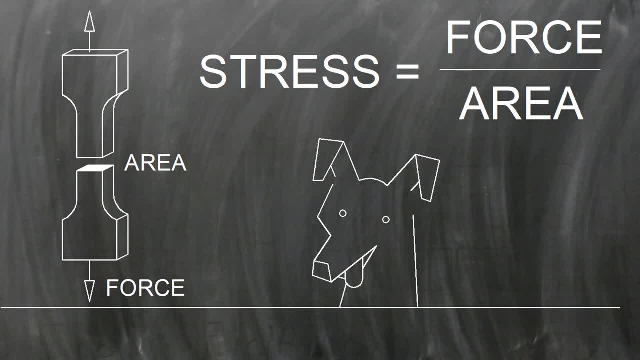 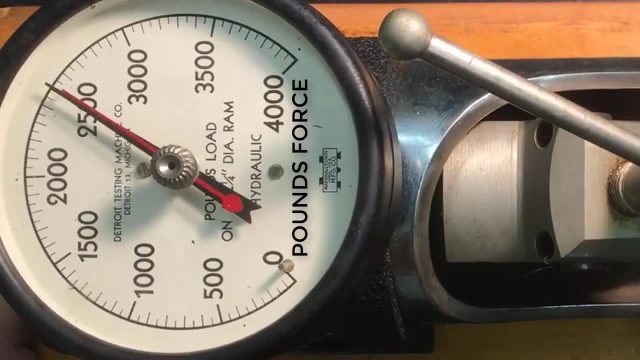 Remember that stress is a force divided by a cross-sectional area. The gauge on our tester gives us values of force in pounds. To get stress values, we'll divide the pounds by the cross-sectional area of the sample. The sample we're going to test is .450 inches. 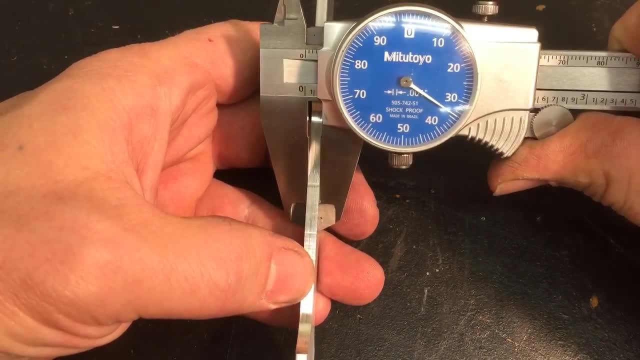 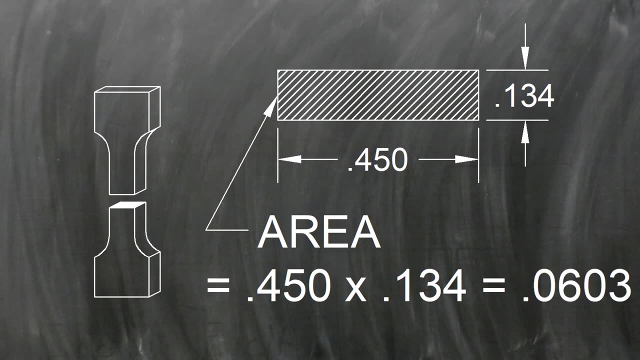 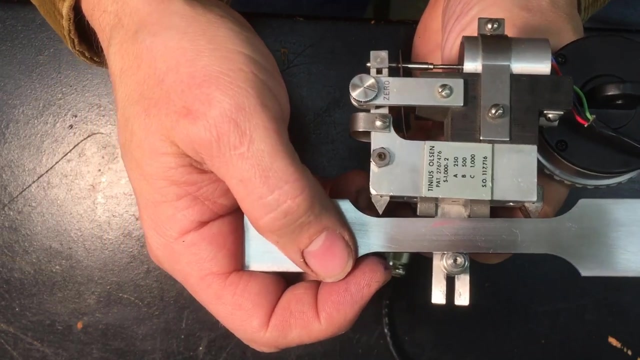 The gauge is wide by .134 inches thick, so the cross-sectional area is .0603 square inches. We'll want to know about strain too. This device, called an extensometer, will measure how much the specimen is stretched. We'll set it so that these knife-edge prongs are two inches apart. 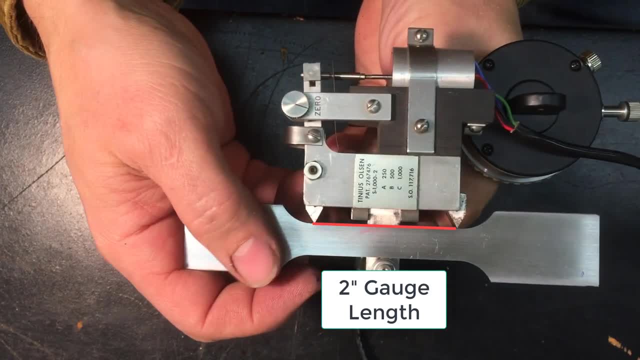 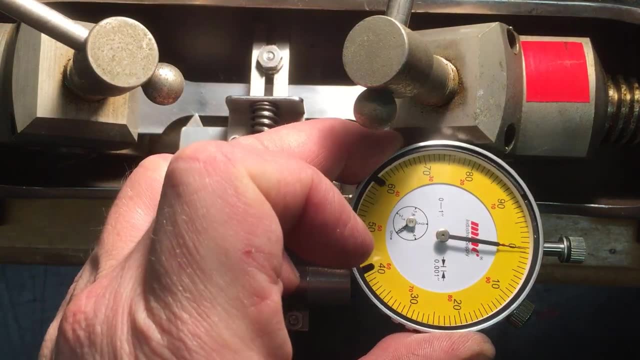 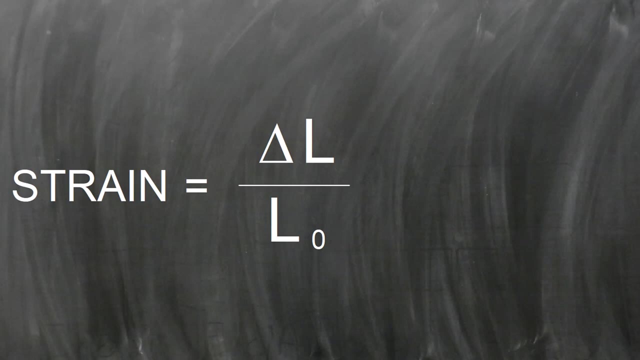 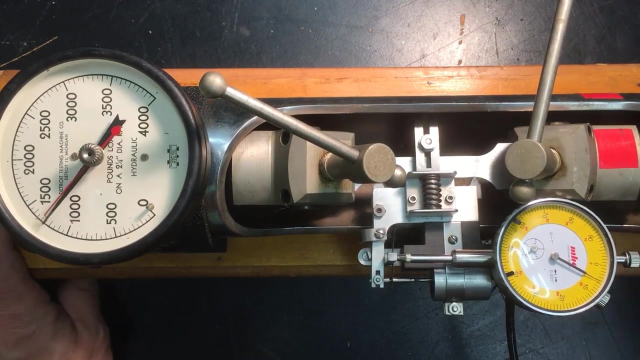 We'll call this the gauge length and this will be our original length. Then we'll measure the amount the dial moves and divide by our two-inch gauge length. Remember that strain is the change in length divided by the original length. Now, as I begin turning the crank, you can see that the value on the force gauge dial 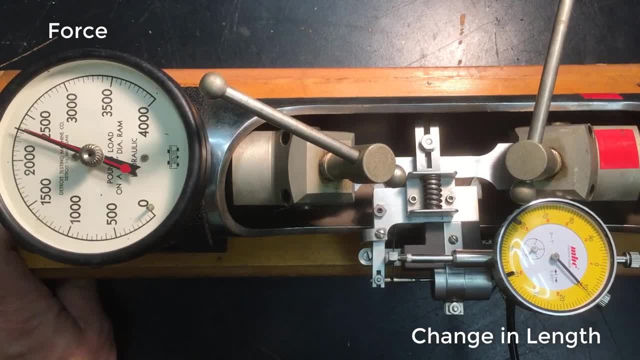 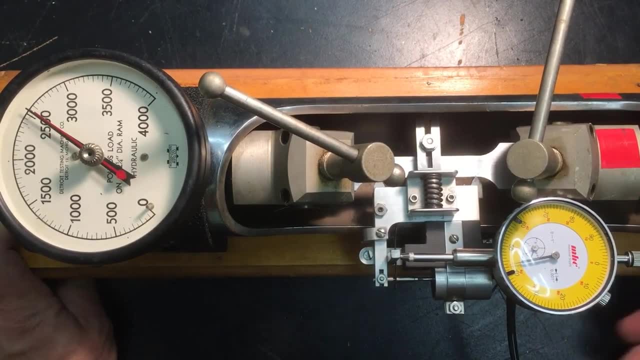 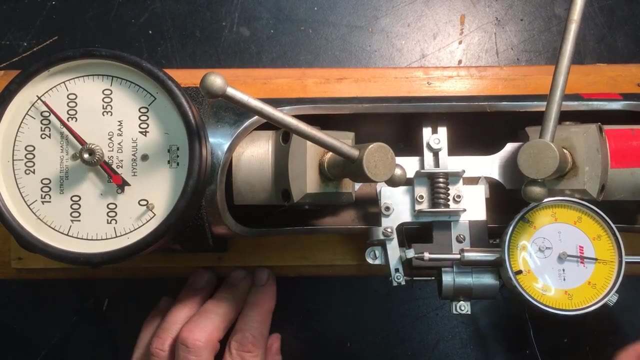 quickly rises, while the dial on the extensometer barely moves. But as I keep cranking, the force gauge dial almost stops increasing and the extensometer starts moving more and more. Eventually the dial on the force gauge drops down a little bit. 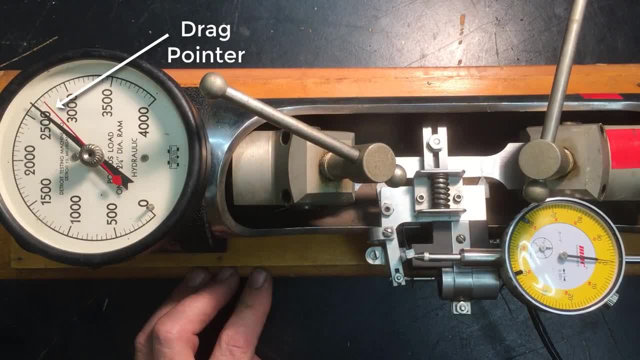 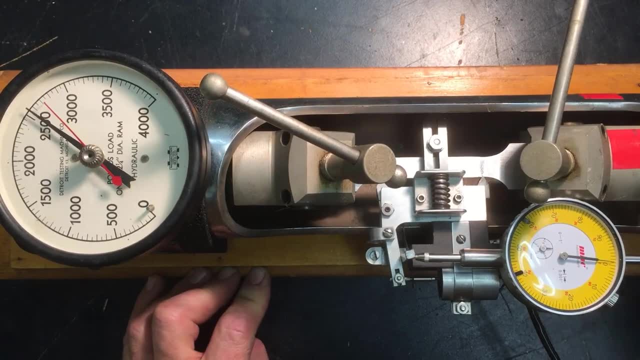 This red drag pointer shows where the force reached its maximum. This drop tells me the sample is about to break, so I'll remove the extensometer so it won't get damaged. As I keep cranking, I can see the sample start to neck down and it breaks. 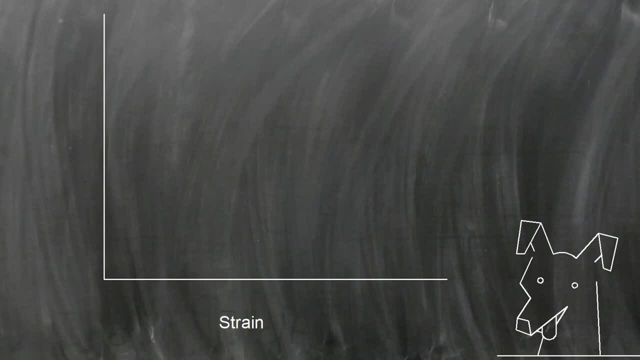 Let's plot this on a diagram. We'll put strain along this axis and we'll label it .500.. We'll label it with a lowercase epsilon or a greek letter E. We'll put stress on this axis and we'll label it with a lowercase sigma or a greek letter S. 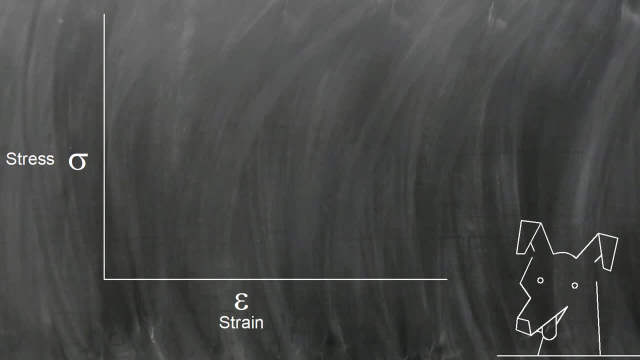 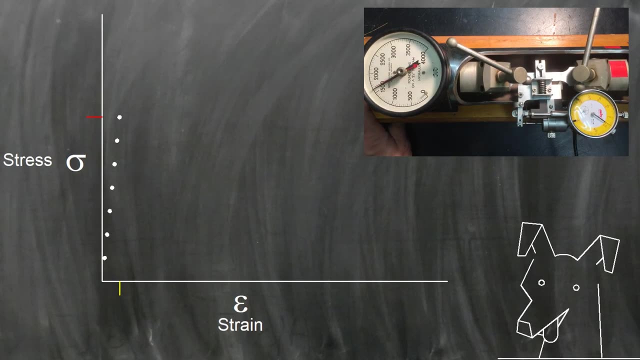 Now let's take some values from our test to see the relationship between stress and strain. When we first began turning the crank to pull the sample apart, the stress built up quickly and there was very little strain. Notice that the graph for this region makes a straight line.